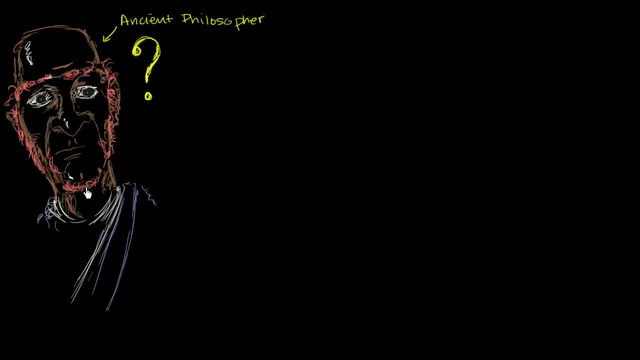 Let's say that you are an ancient philosopher who is building up mathematics from the ground up, And you already have a reasonable understanding of what a negative number could or should represent, And you know how to add and subtract negative numbers. But now you are faced with a conundrum. What happens when you multiply negative numbers, Either when you multiply a positive number times a negative number, or when you multiply two negative numbers. So, for example, you aren't quite sure what should happen if you were to multiply- And I'm just picking two numbers where one is positive and one is negative. 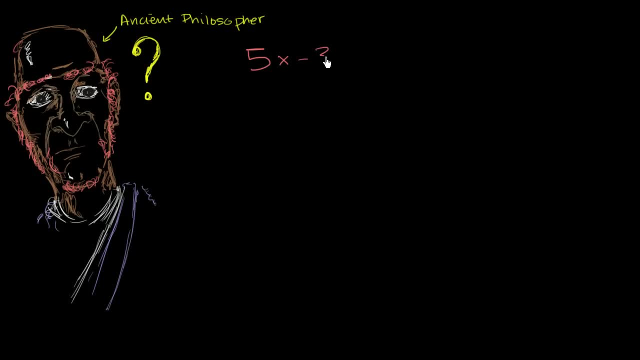 What would happen if you were to multiply 5 times negative 3?? You're not quite sure about this just yet. You're also not quite sure about what would happen if you multiply two negative numbers. So let's say negative 2 times negative 6.. 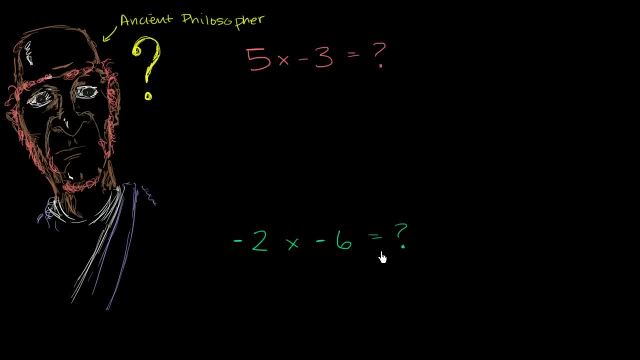 This is also unclear to you. What you do know, because you are a mathematician, is, however you define this, or whatever this should be, it should hopefully be consistent with all of the other Uh Properties of mathematics that you already know. 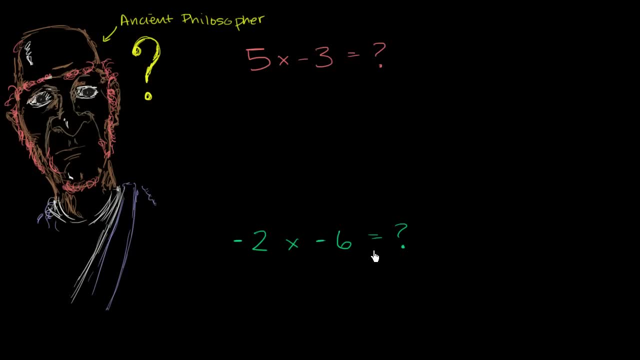 And preferably all of the other properties of multiplication. That would make you feel comfortable that you are getting this right And later we can think about other ways to get the intuition for what these might be and why it actually makes sense. But to make this consistent with the rest of the mathematics that you know, 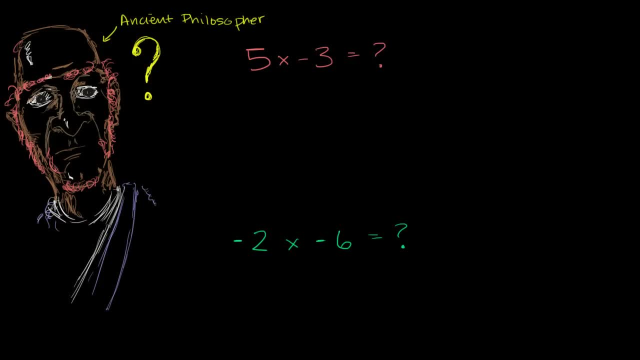 you go into a little bit of a thought experiment. You say: well, what should 5 times 3 plus negative 3 be? Well, you already have. You have a philosophy of adding negative numbers, or adding positive to negative numbers. 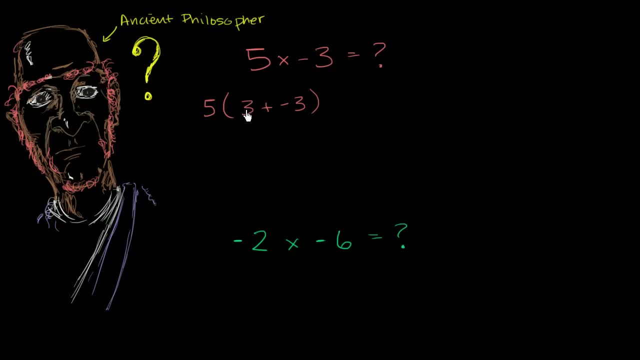 You know that negative 3 is the opposite of 3.. If you add 3 to negative 3, you're going to get 0. So this is going to be equal to 5 times 0, based on how you already thought about adding a negative to a positive. 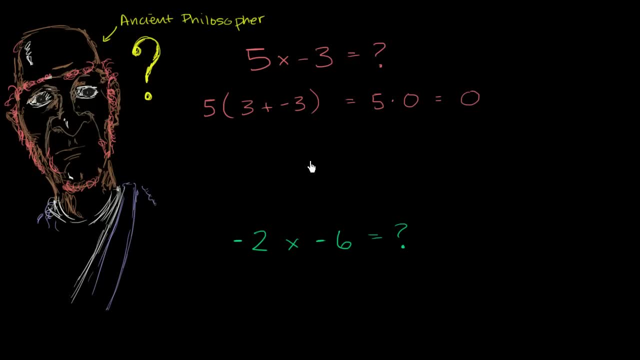 And anything times 0 is going to be 0. So this expression right over here should be 0. But on the other hand you say: well, I want multiplying positive and negative numbers to be consistent with the distributive property. So I should be able to distribute this 5.. 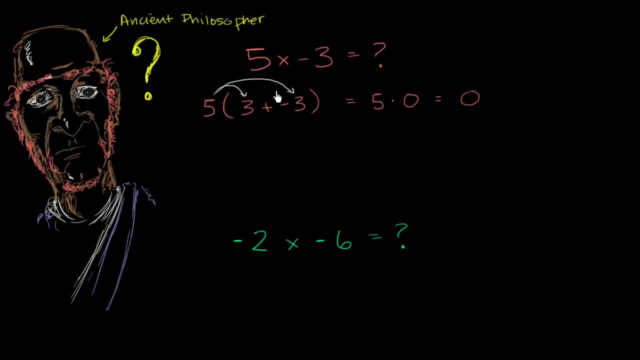 And for math to be consistent- and math should be consistent- I should get the exact same answer. So let's distribute this 5.. So if we get 5 times 3, let me write it out- This is going to be 5 times 3.. 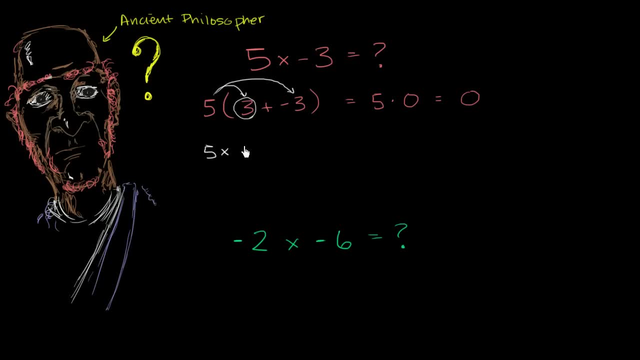 Let me write it with a multiplication, not the dot. I'll write the x sign for multiplying 5 times 3, so I distribute it there plus 5 times negative 3.. And I'll do that in yellow: 5 times negative 3.. 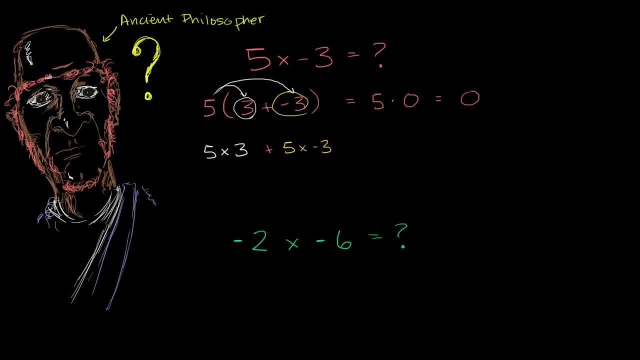 And this whole thing we just said should be equal to 0.. Well, 5 times 3, those are two positive numbers. We know what that should be. That is going to be 15.. So now we get this thing: 15 plus whatever. 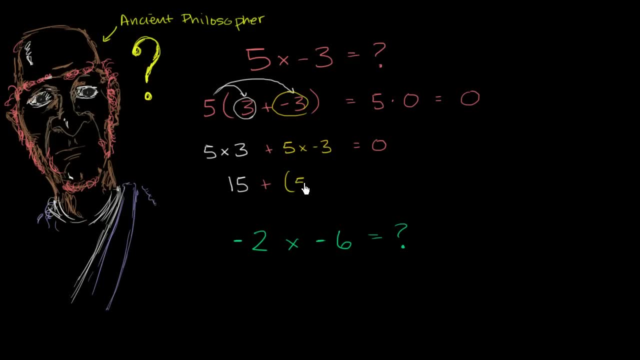 5 times negative 3 is plus. whatever 5 times negative 3 is needs to be equal to 0 in order to be consistent with all of the other mathematics that we know. Well. what plus 15 is going to be equal to 0?? 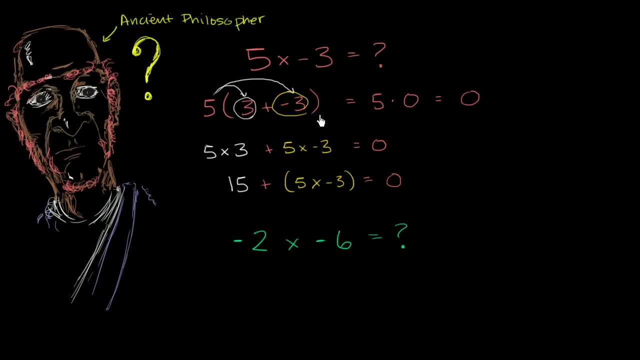 Well, the opposite of 15.. In order for this to be true, in order for this to be consistent with all of the other mathematics- we know this right over here- needs to be equal to negative 15.. And so you say 5 times negative 3, in order to be consistent with all the other. 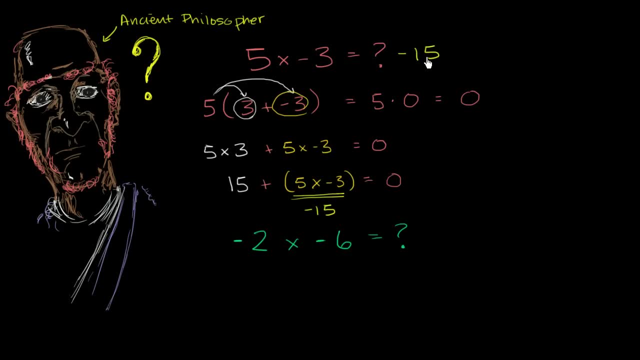 we know, needs to be equal to negative 15. And that's also consistent with the intuition of adding negative 3 repeatedly five times. Now a slightly harder to conceive idea is multiplying two negatives, But we can do the exact same thought experiment. 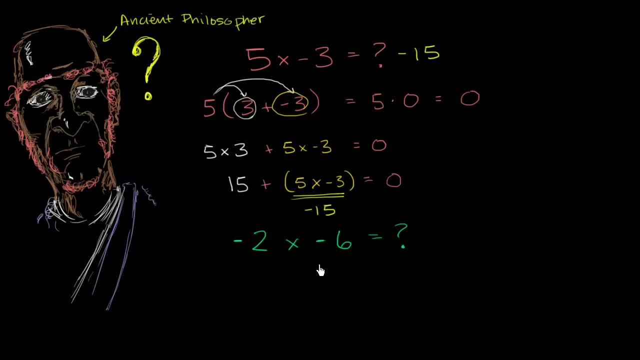 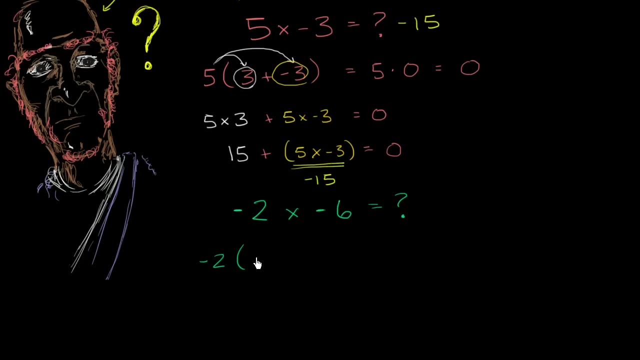 We want, whatever this answer to be, to be consistent with the rest of mathematics that we know, So we can do the same thought experiment. So what would negative 2 times 6 plus negative 6 be equal to? Well, 6 plus negative 6 is going to be 0.. 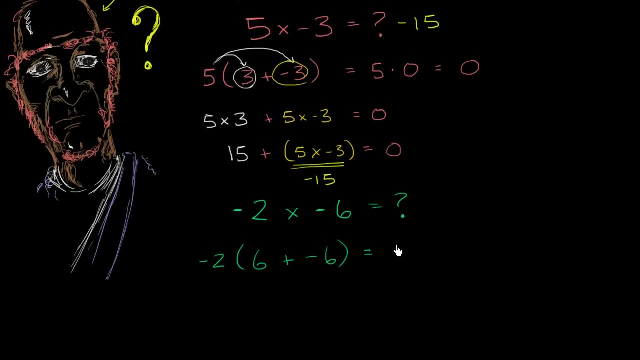 Negative 2 times 0, anything times 0, needs to be equal to 0. But then, once again, we can distribute. We can distribute negative 2 times 6. So we get negative 2 times 6, plus negative 2 times negative 6,. 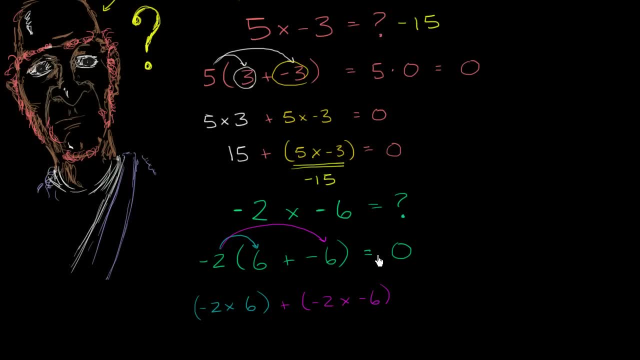 plus negative 2.. Negative 2 times negative 6. And, once again, all of that's going to need to be equal to 0.. Now, based on the thought experiment we just did, we said: well, this needs to be equal to negative 12..